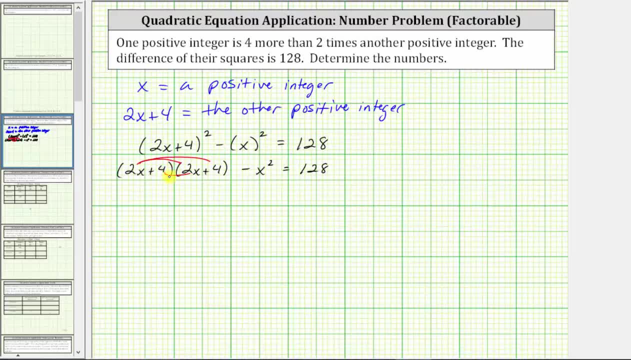 we have four products: One, two, three and four. Two x times two x is four x squared Plus two x times four, that's plus eight x. Plus four times two x, that's plus eight x. And then plus four times four gives us plus 16.. 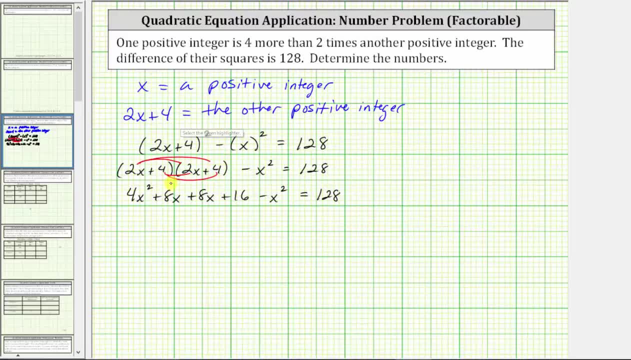 And now we combine like terms. We have two x squared terms and we have two x terms: Four x squared minus x squared, and four x squared minus x squared. 4x squared minus 1x squared is 3x squared. 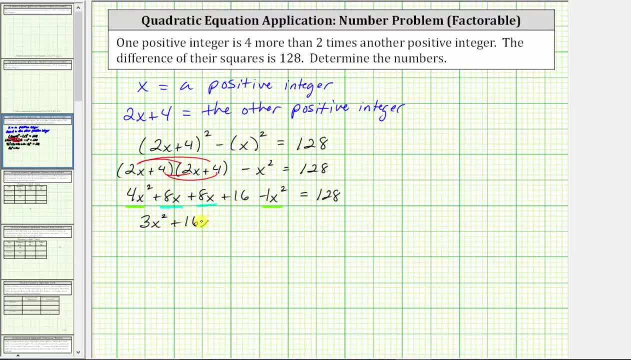 8x plus 8x is 16x, giving us plus 16x. We still have. plus 16 equals 128.. Notice how we have a quadratic equation to solve by factoring. Let's set the right side of the equation equal to zero. 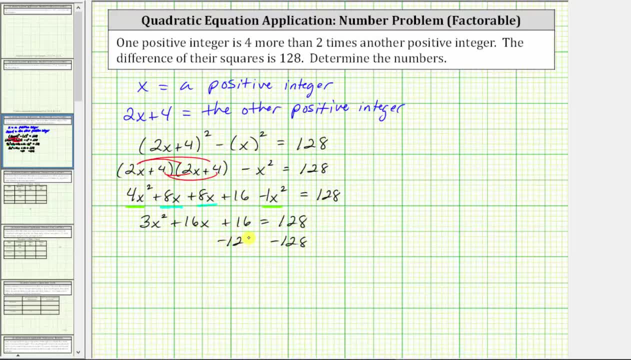 by subtracting 128 on both sides of the equation. Simplifying, we have 3x squared plus 16x. 16 minus 128 is equal to negative 112, giving us minus 112 equals the difference on the right is zero. 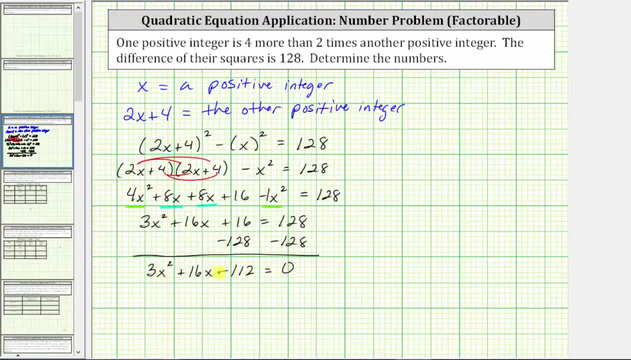 And now we want to factor the right side of the equation. Notice: three is not a common factor, so this will be a challenging factoring problem. If it does factor, it will factor into two binomial factors, Because the first term is 3x squared. 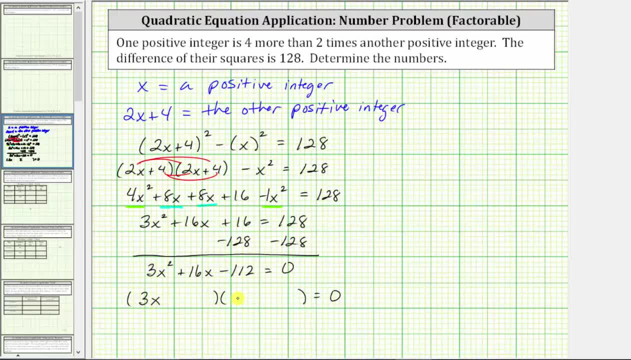 one binomial factor will have 3x as the first term, The other will have x, And now we need to place the factors of negative 112 into the binomial factors so that the sum of the inner product and outer product give us positive 16x. 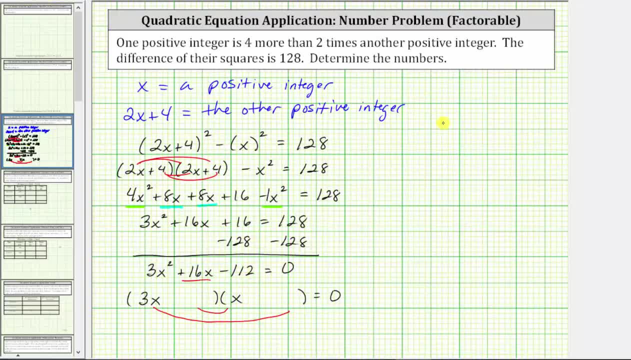 For the next step, let's determine the prime factorization of 112.. 112 is equal to two times 56.. 56 is equal to eight times seven. Eight is equal to four times two, And four is equal to two times two. 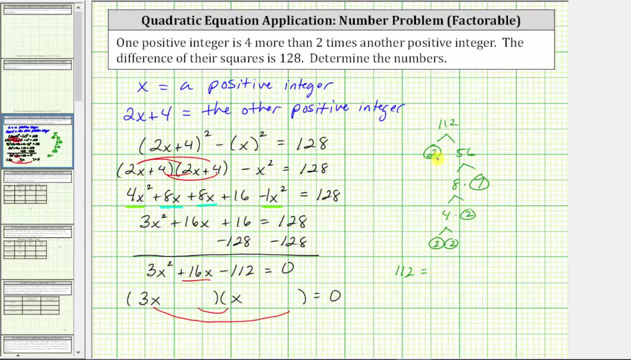 Which means the prime factorization of 112 is equal to one, two, three, four factors of two and a factor of seven. Looking at the prime factorization of 112, notice how two times two is equal to four and two times two times three is equal to four. 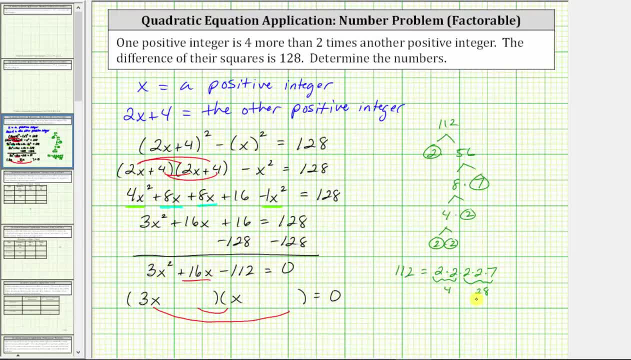 And two times two times seven is equal to 28.. And because we are using the factors of negative 112, we could use negative four times positive 28, or positive four times negative 28 in the second positions of the binomial factors. 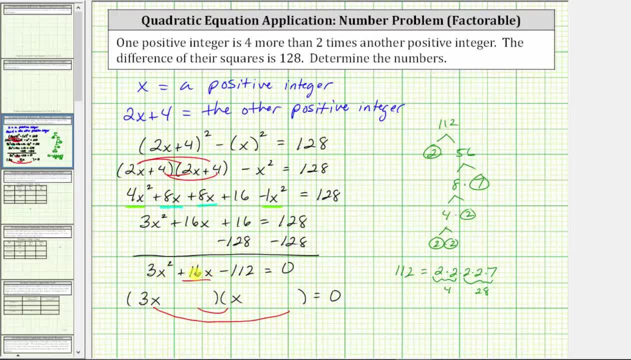 Remember we need the sum of the inner product and outer product to be equal to positive 16.. So let's use positive 28 and negative four and place plus 28 here and minus four here. Let's check to see if this works. 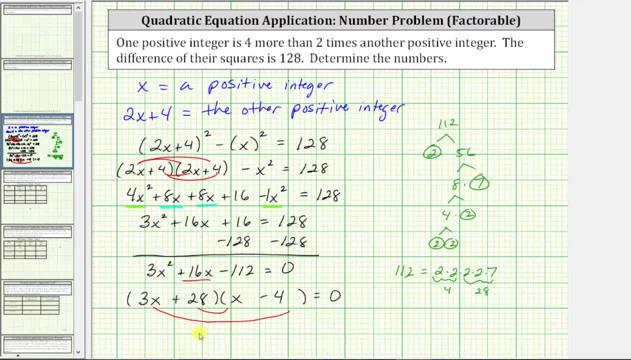 The inner product is positive 28x. The outer product is negative 12x. 28x plus negative 12x is equal to positive 16x, which is a middle term, and therefore we do have this factored correctly. Now that we have it factored, this product is equal to zero. when three x plus two x is equal to zero. Now that we have it factored, this product is equal to zero. when three x plus two x is equal to zero- and therefore we do have this factored- this product is equal to zero. 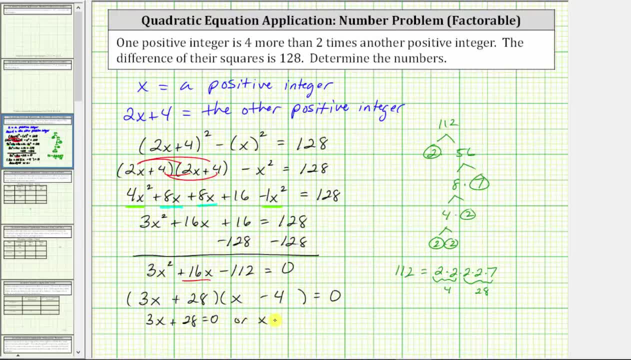 when three x plus two x is equal to zero, and therefore we do have this factored- this product is equal to zero. when three x plus two x is equal to zero, and therefore we do have this factored- this product is equal to zero. 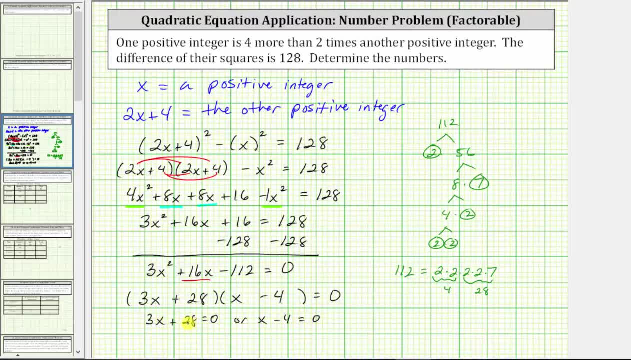 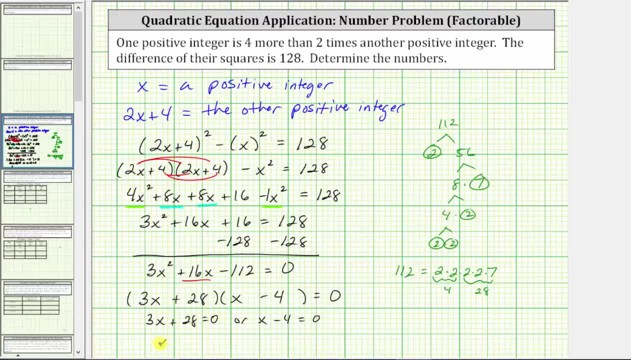 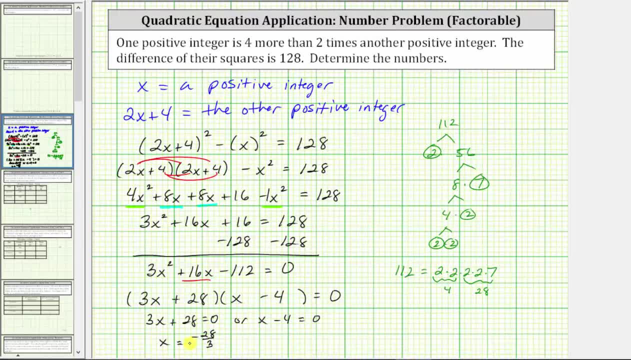 which is not an integer, and therefore we can exclude this as a possible solution. And then, for x minus four equals zero. to solve for x we add four, giving us x equals four. Four is a positive integer and therefore this is the solution that we need. 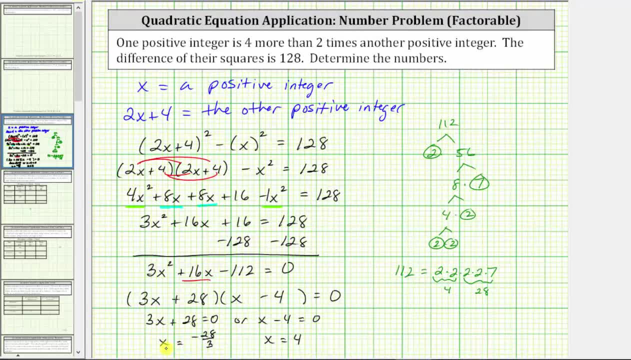 in order to answer the question Again, we exclude this solution of x for two reasons: because it's negative and also it's not an integer Going back up to the top. we now know x is equal to four, so one positive integer is four. 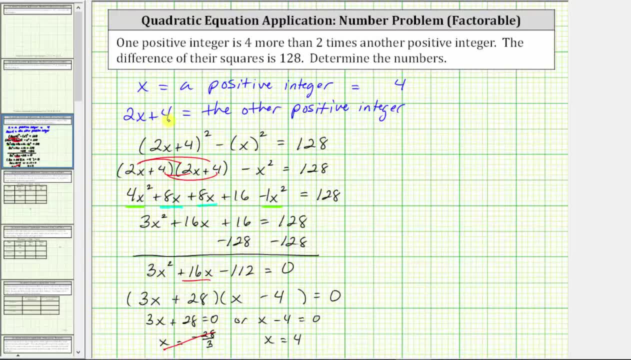 and the other positive integer is represented by the expression two x plus four. so if x is equal to four, we have two times four plus four, which is eight plus four, which equals 12.. Now that we've found the two positive integers, 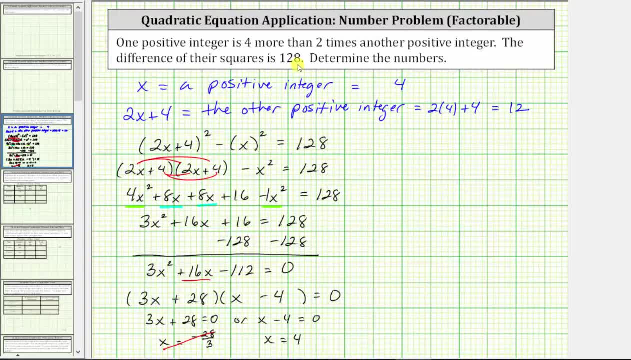 let's just verify: the difference of their squares is 128.. We'd have: 12 squared minus four squared equals 128.. 12 squared is equal to 144.. Four squared is equal to 16.. 144 minus 16 is 128.. 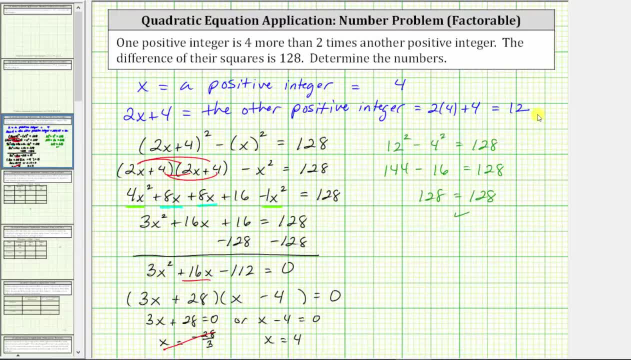 Verifying our solution is correct, Let's write the answer as a complete sentence. The two positive integers are four and 12.. I hope you found this helpful. 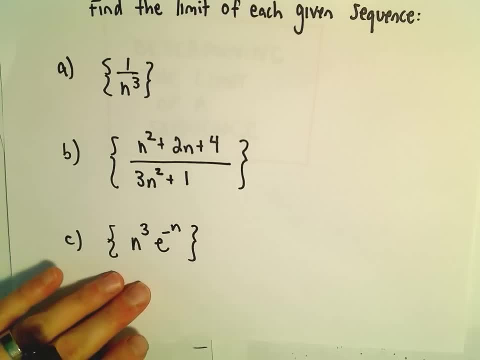 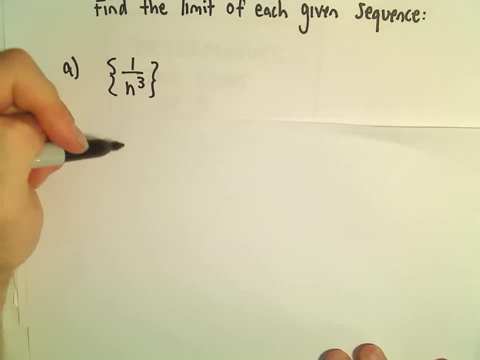 Alright, in this video we're going to look at determining the limit of a few different sequences. So in part A we have the sequence associated with 1 over n cubed. So what we'll do is, again, we just take the limit, as n goes to infinity, of 1 over n cubed. 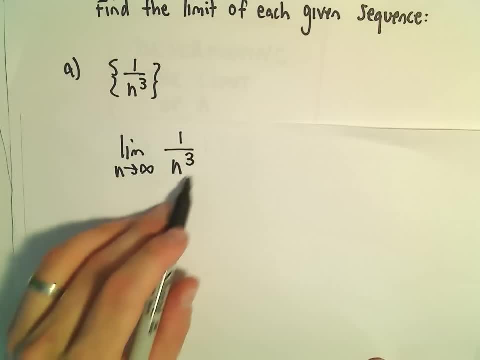 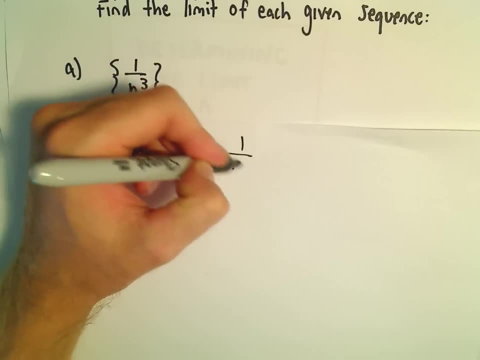 Well, as n gets really really really big, the denominator is going to get really really really big. We're going to have 1 over a very, very big number. So 1 over a large number gets arbitrarily close to 0.. 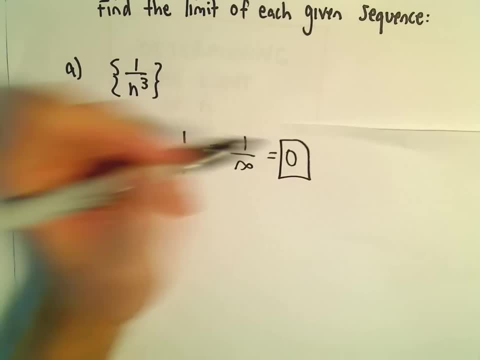 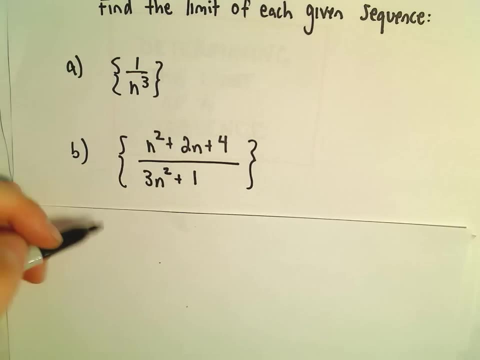 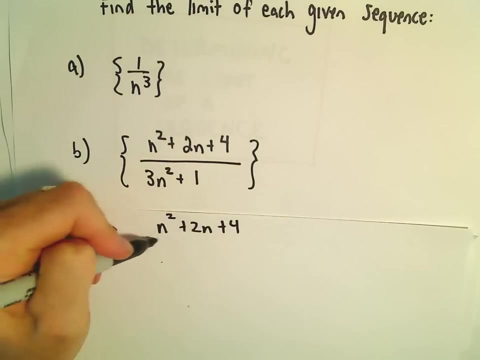 So the limit of the following would just simply equal 0.. Part B: same thing. we'll just take the limit as n goes to infinity. So recall the shortcut. if the degree of the numerator is equal to the degree of the denominator, 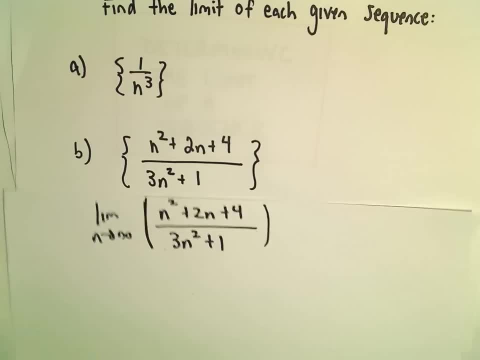 we just do the ratio of the coefficients, So I can just simply look at this and say: well, this is a denominator. This is 1n squared and 3n squared. The degree of the top equals the degree of the bottom. 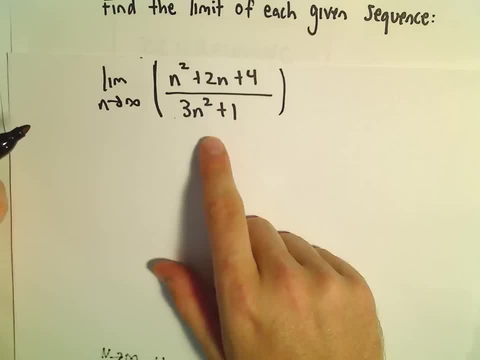 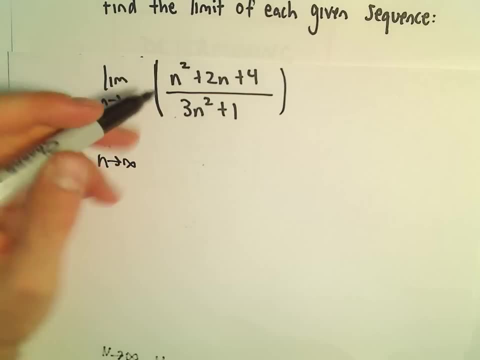 We'll get 1 third. It's a very useful little shortcut to remember when you do sequences in series. But again, kind of to show it with a little bit more work, we can divide everything by n? squared. So n squared over n squared is 1..